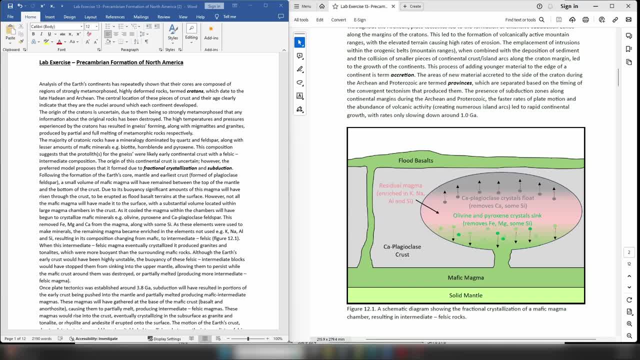 So these cratonic regions are a mixture of gneisses, migmatites, granites and a few lesser rocks along with them. Now, the fact that these rocks have suffered such high degrees of metamorphism and are so strongly deformed instantly suggests that they have been involved in some kind of large 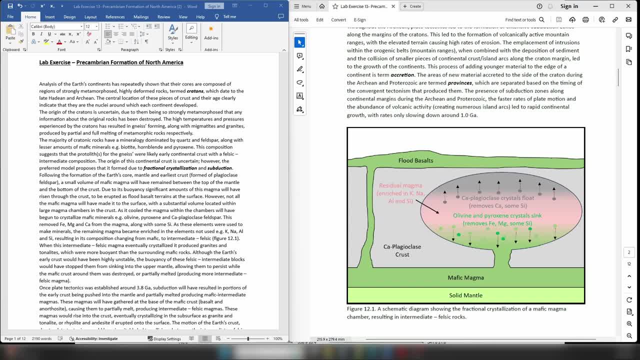 scale collision. So the process that's bringing them together is clearly orogenic in nature, because that would explain why we have these very deformed rocks, because obviously the impact of these two pieces of crust hitting each other Is going to lead to significant deformation. and we also know that the collision of two 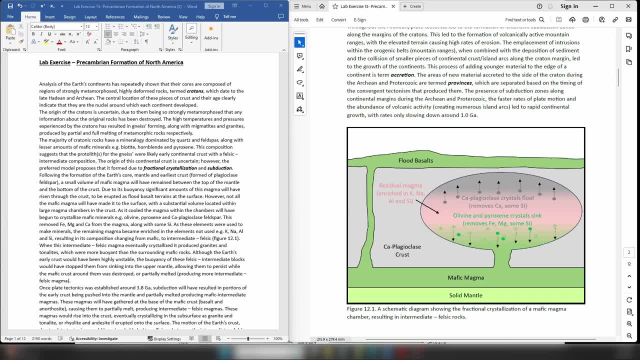 pieces of crust together will typically result in a mountain range, thereby bringing about quite high pressures and temperatures, especially towards the core of said mountain range. Now, the majority of the cratonic rocks are dominated by quartz and feldspar, along with lesser amounts of mafic minerals. 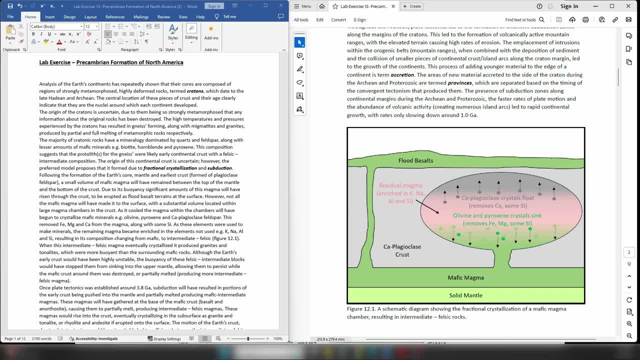 So those would be biotite, hornblender, pyroxene. Now this composition would suggest that the precursor rocks, the protoliths or these cratonic rocks, were probably continental crust. It's uncertain whether you know the rocks we're talking about were granites or whether 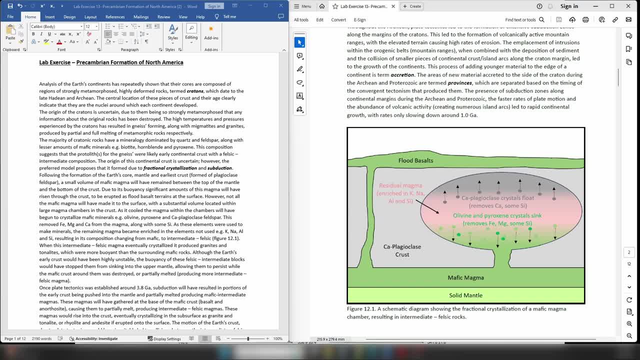 they could even have been sedimentary rocks That you know. that information is no longer around. It's been destroyed by the metamorphism and deformation. but it would seem more than likely that These cratonic regions represent pieces of continental crust that have undergone very 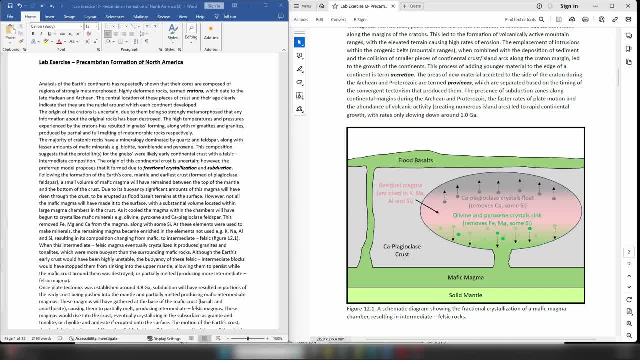 very high levels of deformation and metamorphism during the Archean and into the early Proterozoic. So the origin of continental crust itself is somewhat uncertain. So if you remember, when the earth was first crystallizing from the magma ocean, we ended up with a crust that was made up of anode. 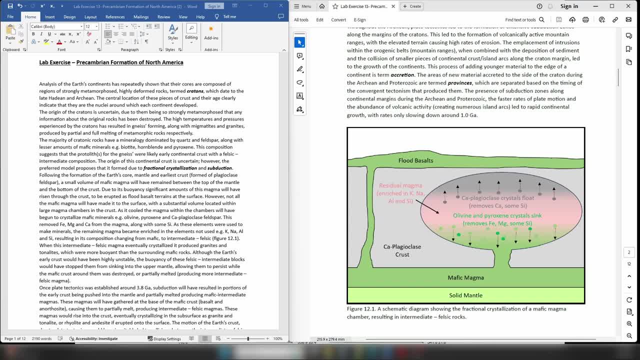 So we had an anorthosite crust that would have been quite light in colour and it would have looked relatively similar to the highlands of the moon. So the question then becomes: well, how do we go from that kind of crust to the formation of pieces of continental crust? 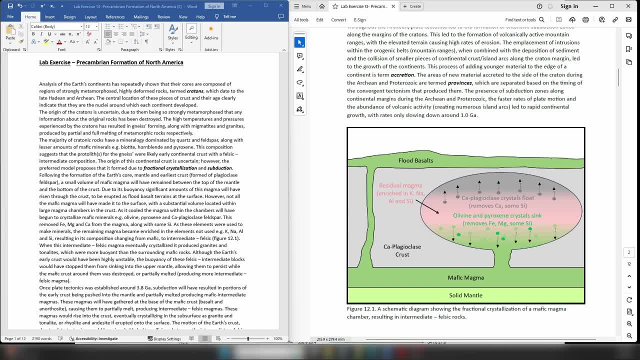 So there's a couple of ways that we can do it. So we can do it through fractional crystallization and we can do it through subduction. So we know that as the magma ocean was cooling, We first formed the earth's core, then we started forming the earth's mantle and then 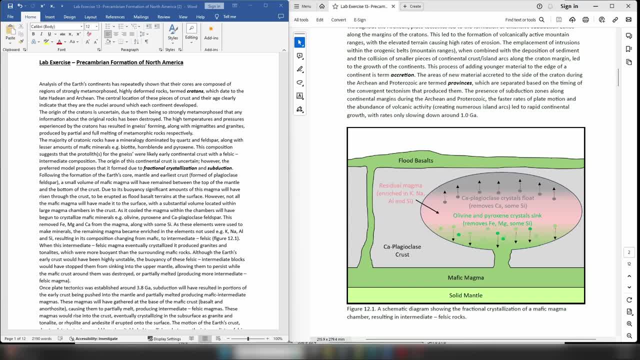 we started forming this anorthite rich crust And steadily over time, as the magma ocean cooled down, obviously the constituents of that magma were steadily turned into solid minerals and those solid minerals became part of the mantle or the crust. Now, what you have to remember is that during the process of forming new minerals, you are 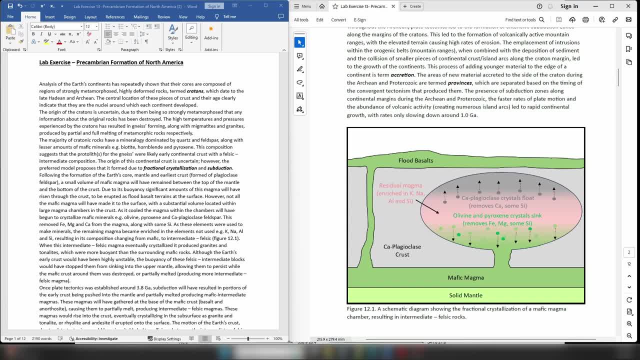 using up elements from the magma. Those are typically referred to as the compatible elements, because they are compatible with the minerals which are crystallizing. That also therefore means that you have elements which are not entering the minerals crystallizing. These are incompatible elements and so, for instance, if you were crystallizing out, let's 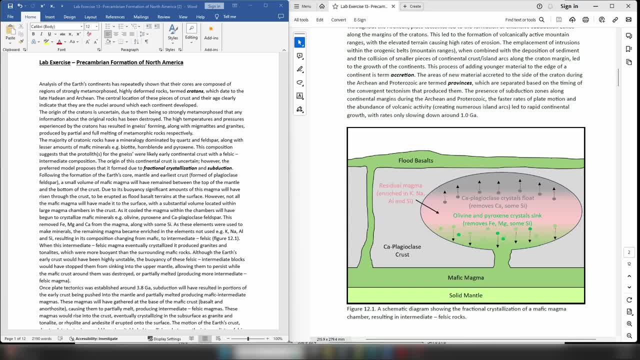 say pyroxene and olivine, well, you would be removing magnesium and iron and calcium and a bit of silicon. You would be removing magnesium from the magma to make those minerals, but you would not be using things like sodium, potassium and aluminium So steadily over time as the volume of magma decreases because it's being turned into solid. 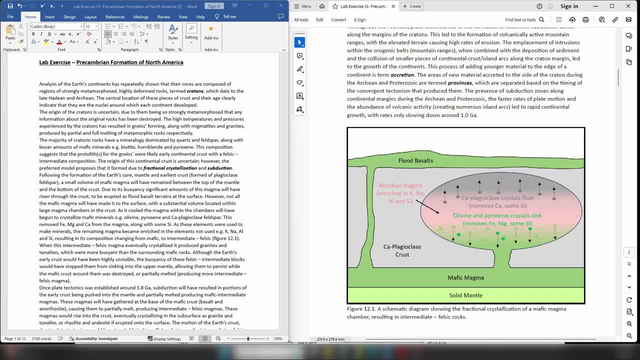 minerals. you end up with a residual magma that steadily becomes richer and richer in these incompatible elements, And so, eventually, what we end up with is a situation where we have the mantle and we have this anorthite rich crust, And then, stuck between the two of them, we have this layer of quite strongly fractionated 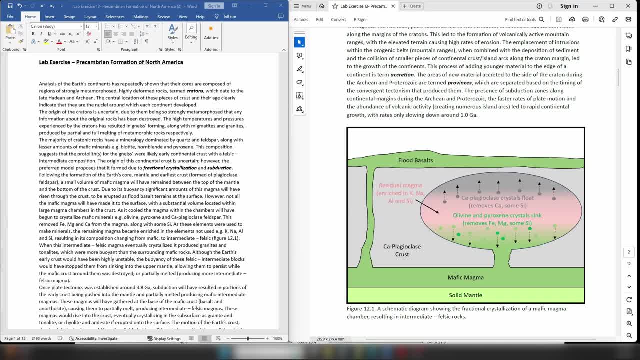 magma, And this magma is going to have a composition which is going to be sitting somewhere around mafic, maybe even intermediate. And so what's going to happen is this magma is naturally going to want to rise. It's hot, it's buoyant, it's going to want to go up. 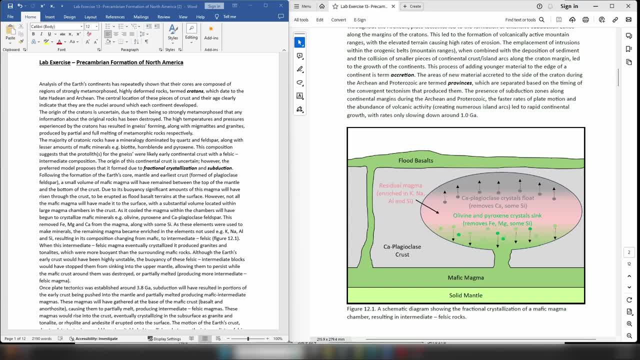 And because this early crust is typically going to be quite unstable, There are going to be plenty of opportunities for some of this magma to rise up into the early crust Now. some of it will make it all the way to the surface, where it will be erupted as flood. 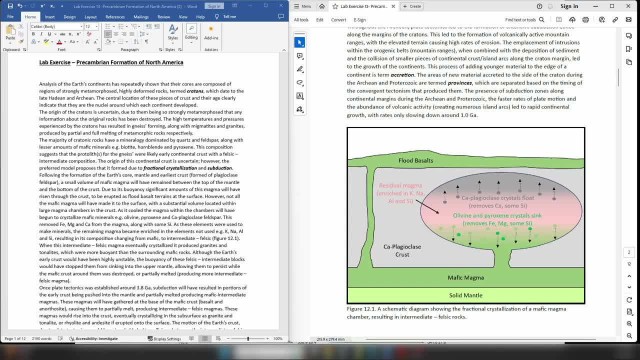 basalts, But a significant portion of it will not make it to the surface and it will become trapped and it will form magma chambers. Now, on the right hand side over here, we have a schematic diagram of the kind of situation that we envisage occurring. 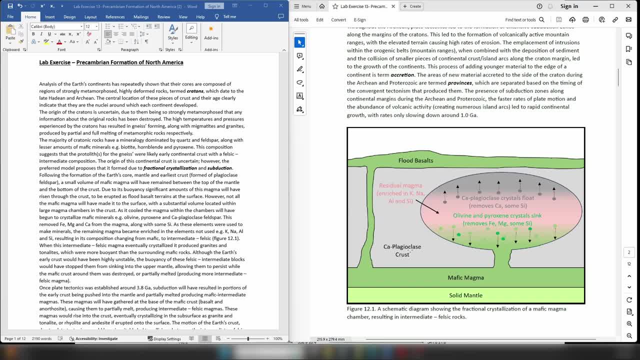 So we have our crust here Included In grey made of calcium, plagioclase, feldspar or anorthite, And we have our solid mantle down here in the light green, and between the two we have this residual mafic magma. 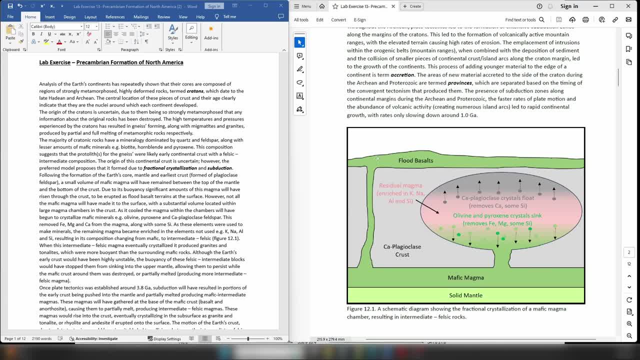 Now, as you can see, some of this magma will be able to make its way through the crust and it will be erupted onto the surface as flood basalts. However, there's also going to be this significant portion that gets stuck in the crust, where it forms magma chambers. 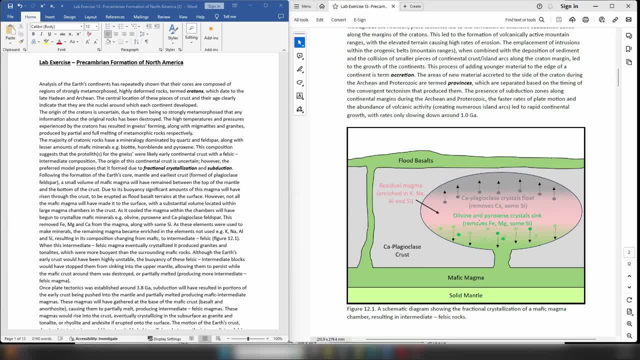 Now these magma chambers are initially going to start off with a mafic composition, approximately, And what's going to happen is steadily as olivine and pyroxene forms, iron, magnesium and some silicon is going to be removed from the magma within the magma chamber. 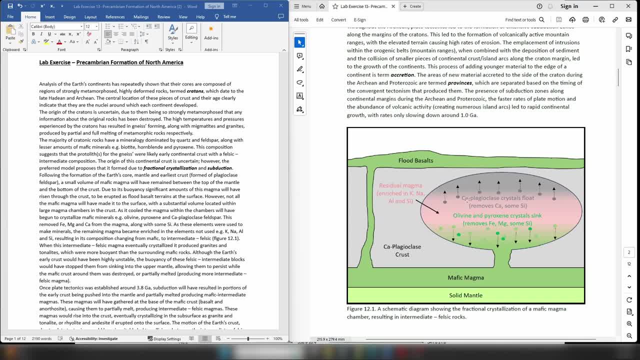 At the same time, we are also going to have calcium being removed in the form of calcium plagioclase feldspar, And so this means, steadily, over time, the volume of magma in your magma chamber keeps getting smaller and smaller and smaller, and, as we've discussed, these incompatible elements will. 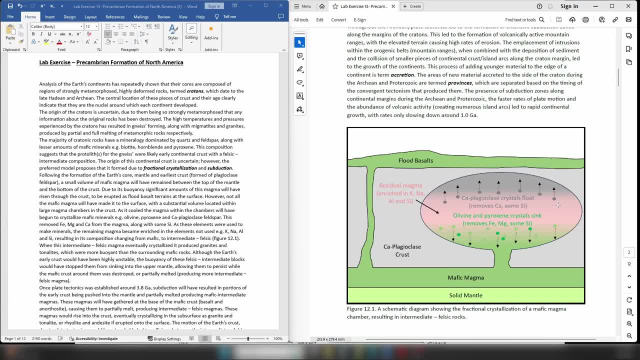 begin to concentrate in this residual magma. So this residual magma here will start to become richer in things like sodium, potassium, aluminium, silicon, you know even stuff like uranium and thorium and yttrium and zirconium, and there's a whole range of elements which are not going into minerals like olivine and 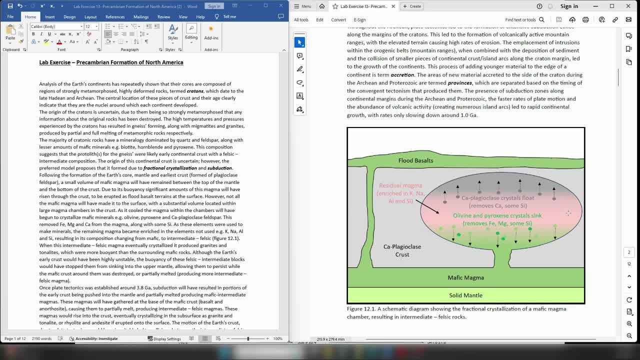 pyroxene or calcium, plagioclase, feldspar, and so they end up fractionating, getting retained within this residual magma, And eventually this residual magma will start to become rich in things like sodium, potassium, aluminium, silicon. The composition of this residual magma is going to move into the intermediate range. 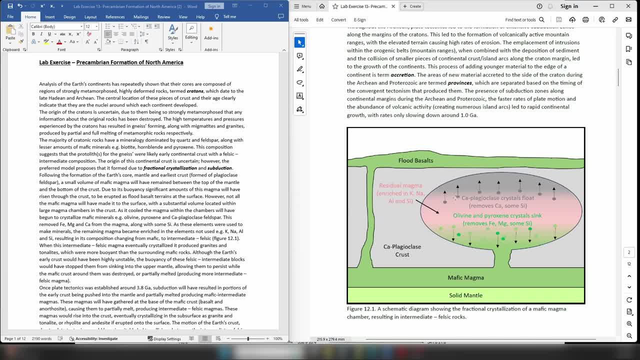 and over time, if it stays liquid for long enough, it will eventually develop a felsic composition, And so what this means is, within these magma chambers, you not only have a whole load of ultramafic rocks and a whole load of mafic rocks, you are also going to have blocks of 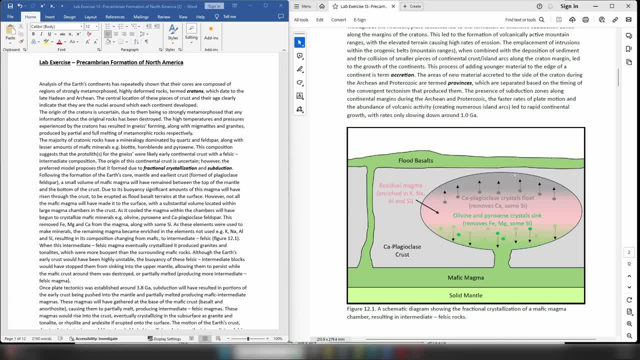 intermediate and felsic plutonic igneous rocks. so you're going to have tonalites and granites. Now you're also going to have a lot of magma. Now you're thinking to yourself: hold on a minute. one magma chamber isn't really going. 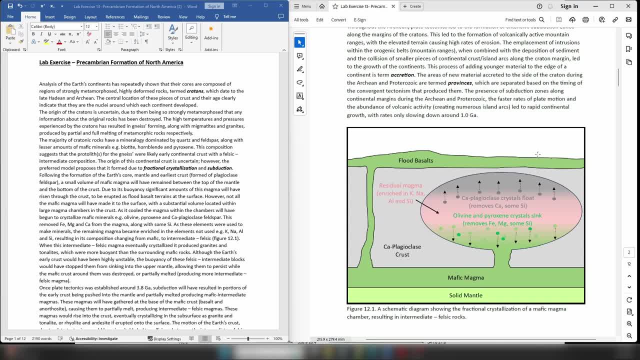 to be enough, and you are correct about that. however, typically weaknesses get repeatedly exploited by rising magma, So your magma chamber may form and then, a few million years later, bang. another magma chamber is going to, another pulse of magma is going to come up along the same weakness. 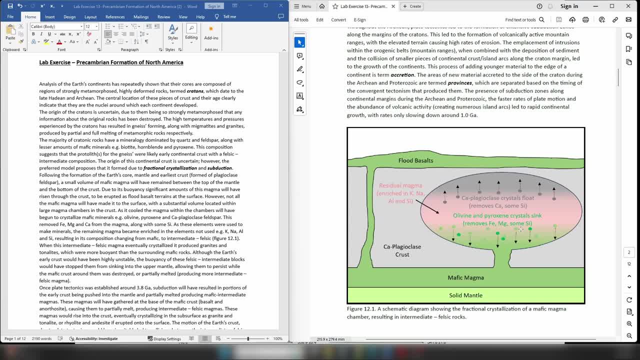 form another magma chamber, and so on, and so on, and so on, and this process will be repeated again and again, and again. And so, over time, this process will be repeated again, and again, and again. And so, over time, this process will be repeated again and again, and again. 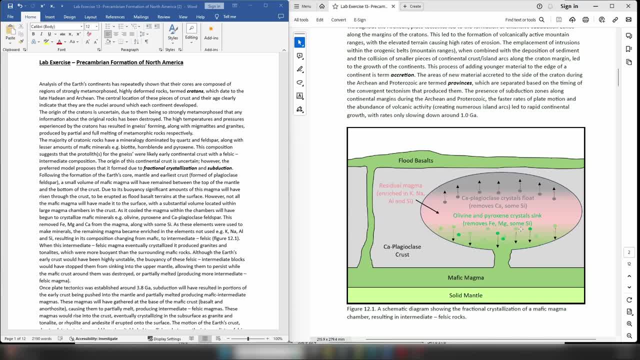 And so, over time in an area, what you end up doing is you end up building up this reservoir of this felsic and intermediate plutonic igneous rock, And obviously we also touched on this in the past when it comes to plate tectonics. 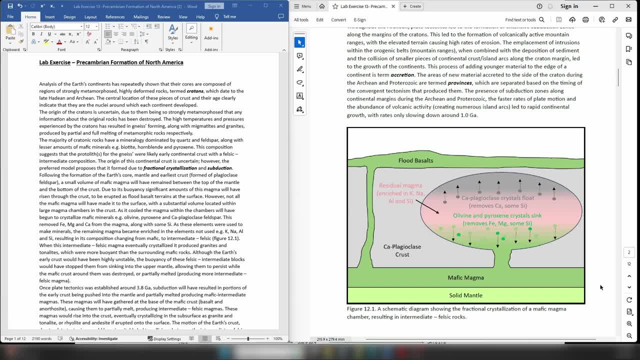 intermediate and felsic igneous rocks are quite difficult to subduct. So that means when plate tectonics really starts kicking in, the more mafic crust is going to start being destroyed. These regions which are richer in felsic and intermediate rocks are going to be more buoyant. 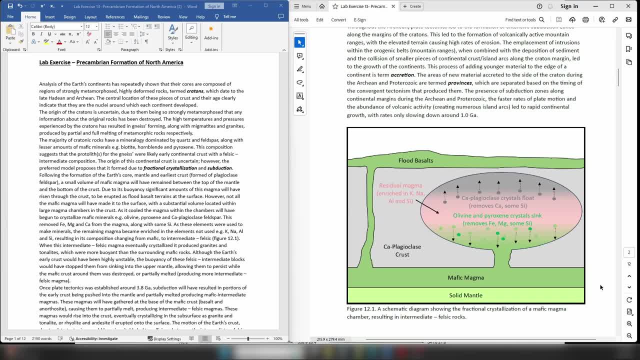 and therefore more difficult to subduct and destroy, And so, over time, they're going to start surviving the subduction process, and so they are going to start moving towards each other eventually, and they're going to start hitting each other, resulting in orogenies. 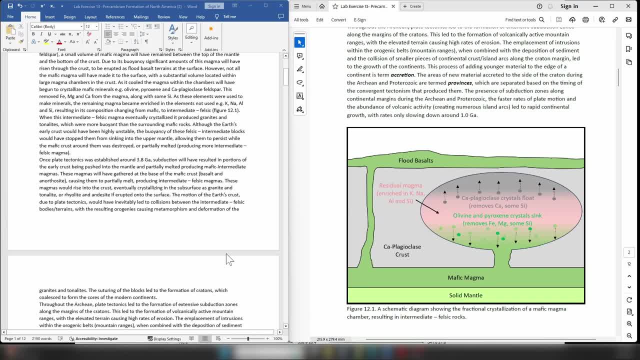 Now the other way that we can start forming continental crust during the Earth's early history is through plate tectonics. Now we know plate tectonics must have been established by about 3.8 billion years ago, And we know this from the issue of Greenstone Belt in Greenland. 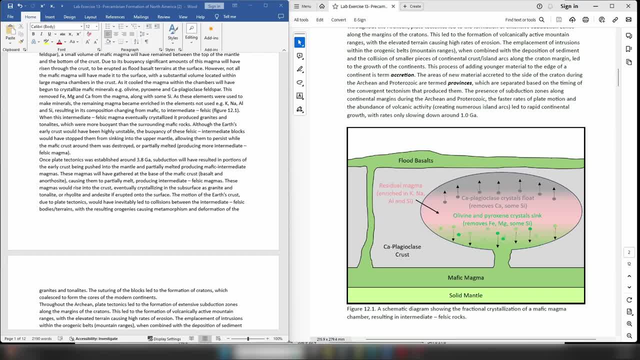 And this is an example of obduction. So that's when oceanic crust has been pushed onto the continental crust. Now, the fact that obduction has occurred means that there must be some force which is pushing the oceanic crust onto the continental crust. 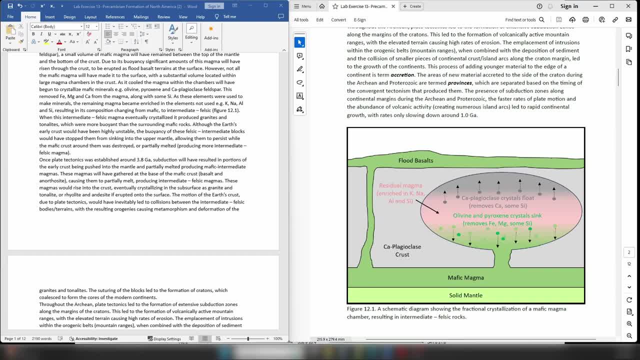 So therefore, we know plate tectonics. Plate tectonics must have been active at that time And we also therefore know where we have obduction. there will also be subduction. So we know that by 3.8 billion years ago, subduction was occurring. 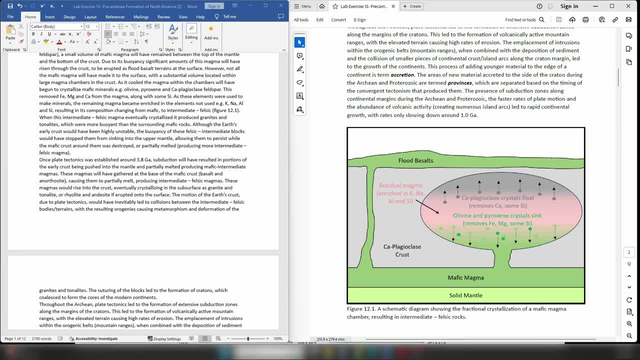 Now, to be clear, it was not easy subduction. It's not like the subduction now. What you would have been dealing with is relatively young, warm, mafic crust, so basalts and maybe some anorthosites. So they're hot and so they're not naturally going to want to sink. They don't have a load of sediment on top of them pushing them down like modern oceanic crust does, So that makes them more difficult to subduct And on top of that, if you do manage to start making them subduct, you have a situation 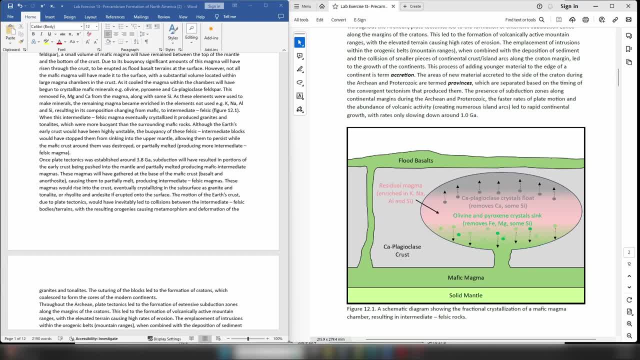 where the mantle they're trying to subduct into is also hotter and more buoyant, So it's more resistance to these pieces of crust pushing down into it, And so this means that early subduction- You know, around 3.8 billion years ago- will have been tricky. 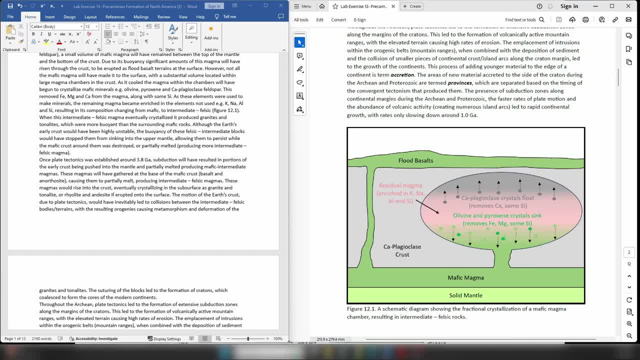 It won't have been an easy process. However, it will have been taking place, And this means that, as we start to subduct these pieces of what we would classify as oceanic crust- so mafic crust- they're eventually going to go down into the mantle and they 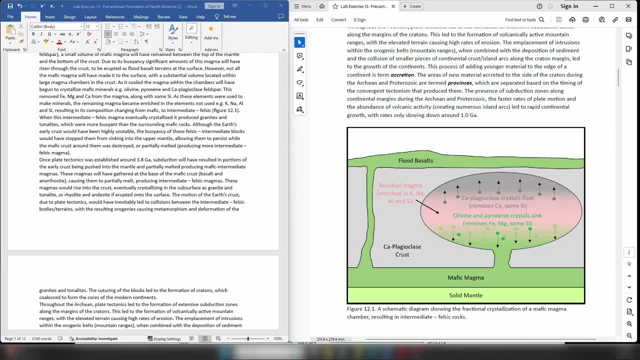 will start to partially melt, And so this crust will partially melt and it will follow the standard procedure: It will form a mafic magma. This mafic magma will then rise up and it will get stuck beneath the bottom of the crust. 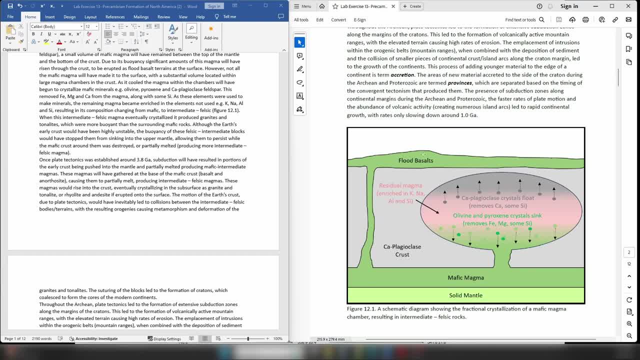 And some of that mafic magma will then enter the crust, where it will crystallize, forming magma chambers like the one we described earlier. However, we also have a situation where the heat from that magma which is trapped at the base of the crust will begin to partially melt the crust in which is you know which? 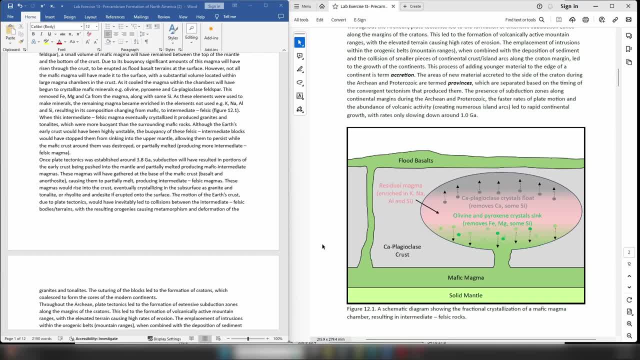 is in contact with. So it might be in contact with mafic crust. So You might have a mafic magma in contact with mafic crust, but the heat from that mafic magma will start to melt some of the lesser minerals within your mafic crust. 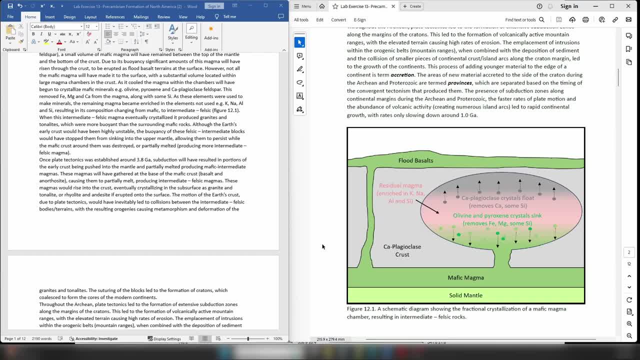 So the small crystals of things like volcanic glass and quartz and feldspar will begin to melt due to the heat from this mafic magma And that will produce a magma which has an intermediate to felsic composition, Because you're melting minerals which are rich in things like silicon, aluminum sodium. 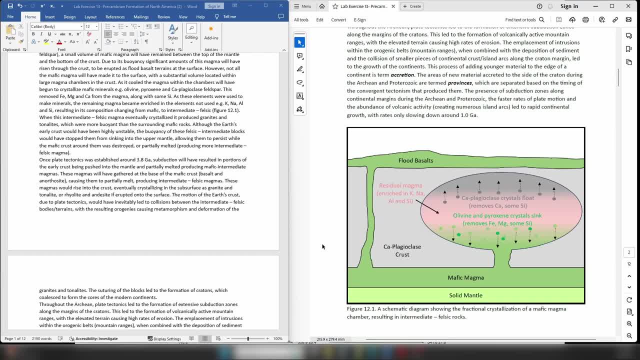 and potassium, the building blocks of a felsic and intermediate magma. So this process of subduction is going to lead to the formation of felsic and intermediate magmas as well, And we know from the modern world that the magmas produced by this subduction process 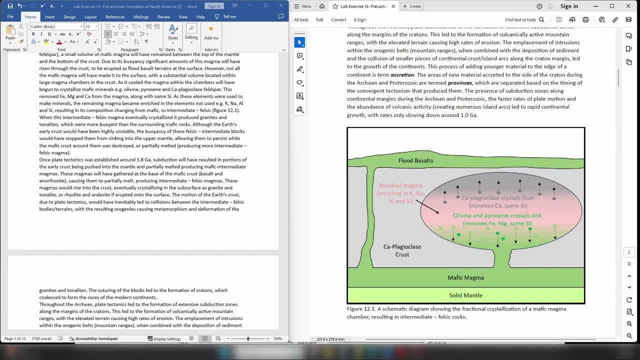 are typically going to rise to the surface, where they will be erupted as volcanoes. So think of the classic example of the Andes mountains: Extremely volcanically active, Lots of volcanoes erupting, intermediate and felsic igneous rocks, And so subduction is going to result in large amounts of intrusion, and these intrusions 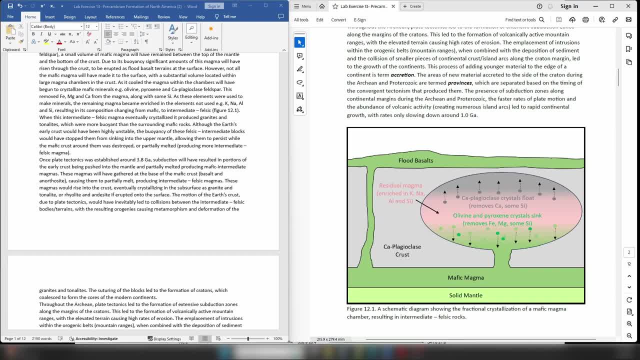 are going to form felsic and intermediate rocks, so granites and tonalites, And then on top of that, we are going to end up with an abundance of volcanoes at the surface as well, which are also erupting intermediate and felsic lavas onto the surface again, creating 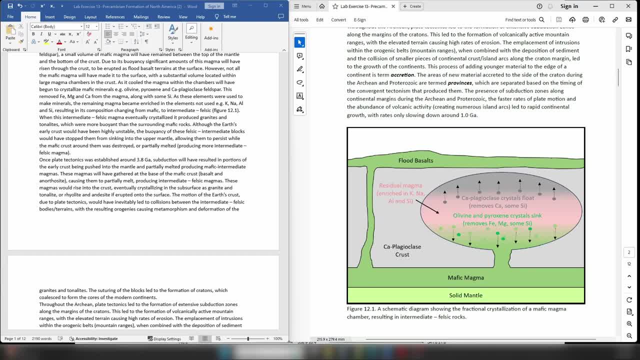 more of these felsic and intermediate igneous rocks. So you can see how a combination of intrusions into the crust and subduction is going to steadily start building up little blocks of felsic and intermediate crust. And so what's going to happen after that? 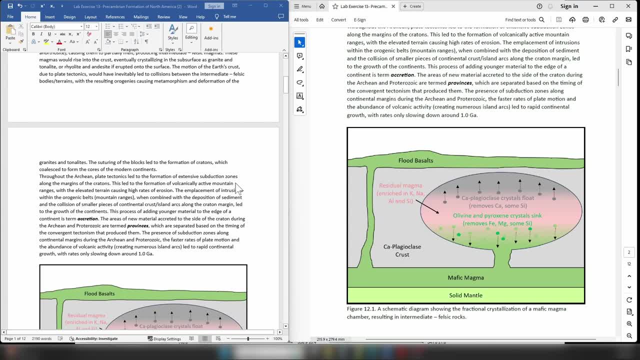 Now We know that during the Archean, The Earth's interior, The Earth's interior, The Earth's interior was considerably hotter And this would have led to pretty chaotic plate tectonics, but it would have also meant that the plate tectonic processes would have been occurring a lot faster, because of all. 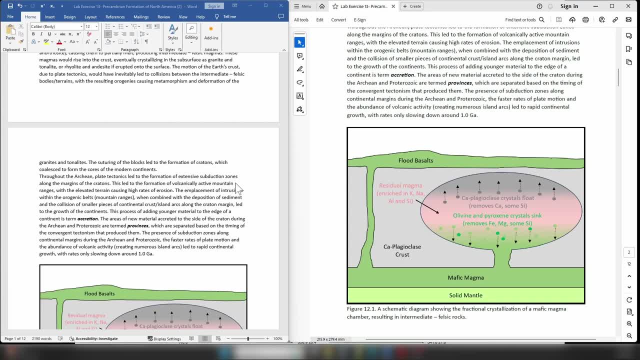 that heat will be driving the systems that allow plate tectonics to take place at a much higher rate, And so this means that these pieces of intermediate and felsic rock, these domains, will be moving around on the surface of the Earth. 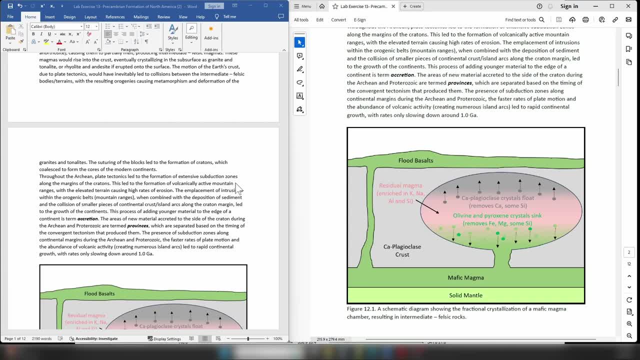 And so they're going to eventually start Banging into each other. And when they do start banging into each other, it's obviously going to start resulting in aroginies. These little microcontinental pieces of granite and tonal light start smashing into each other. 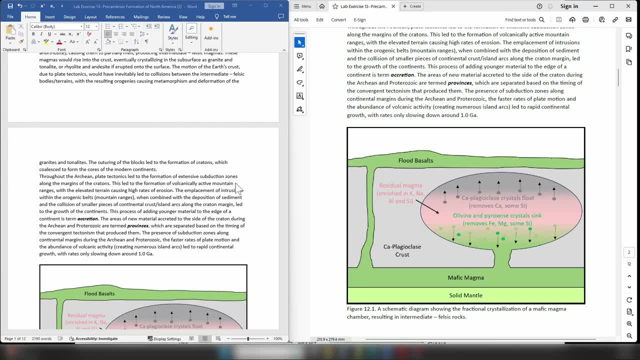 They begin to form larger and larger pieces of crust, They begin to change from just being domains and terrains And they eventually start to combine through collision and eventually they form these microcontinent sized pieces. And these microcontinents are going to be then moving around the surface of the Earth. 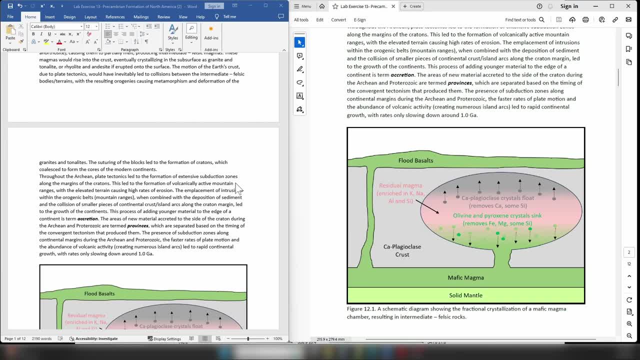 and they're going to keep banging into each other. And this is when we start seeing all this defamation and very high grade metamorphism taking place, Because once you have big enough pieces of continental crust, when they hit each other, they hit each other with a lot of force. 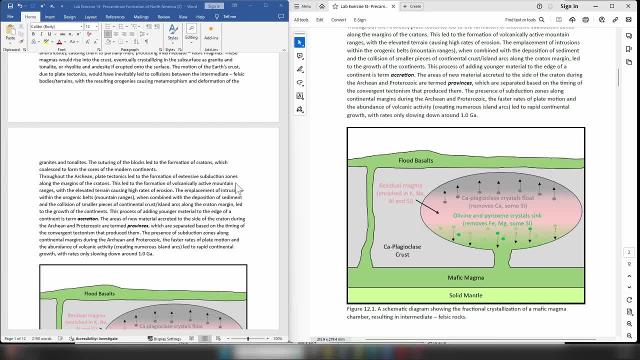 And this is obviously going to result in substantial orogenic events. So you're going to end up building mountain rocks, You're going to end up building mountain ranges which are going to be volcanically active, And so that's going to lead to lots of metamorphism. 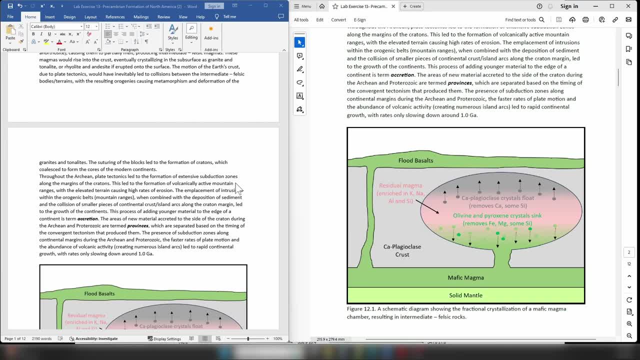 It's going to lead to lots of defamation, There's going to be lots of volcanic activity And there's also going to be some partial melting associated with the collision, So okay. so I hope that gives a general overview of where these pieces of continental crust. 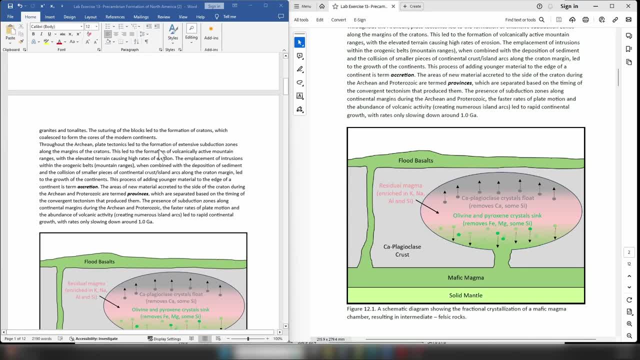 are coming from in the very, very late Hadean and during the Archean. I should point out, by the way, that the majority of the collisions that I'm talking about between these pieces of granite and tonalite rich crust they're going to be mostly taking. 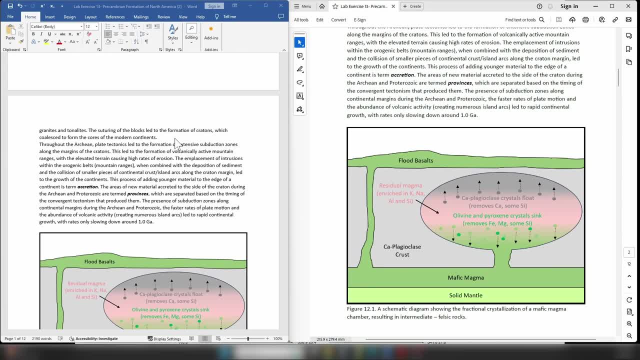 place in the late Archean and early Proterozoic. So okay, so we've ended up with a situation now where we have an abundance of these microcontinents and some of them have hit each other to form even larger continental masses. 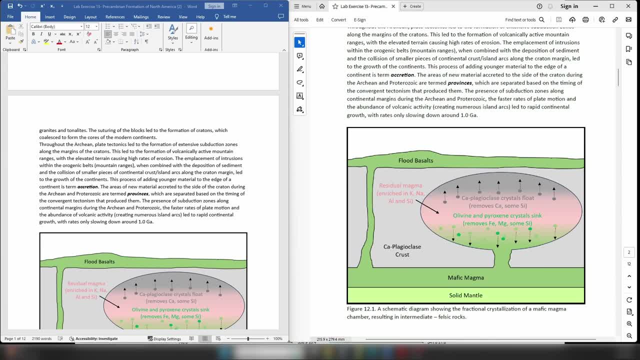 And these are going to become a major problem. So we're going to end up with a situation now where we have an abundance of these microcontinents and some of these microcontinents have become a big problem within our hermitage region At the edge of the. 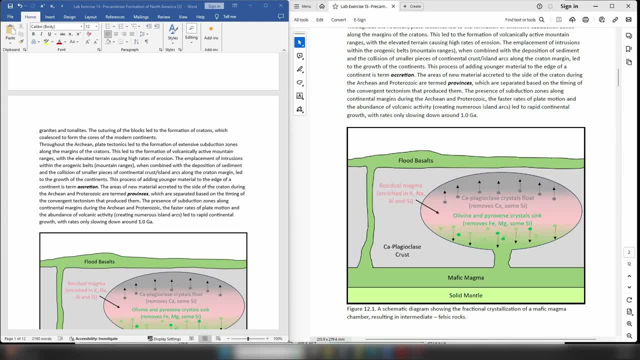 That's where the So the question is is: well, why do we have this racket to look simultaneously? Well, it's all to do with the process of accretion. so Once you formed your craton, your core of your continent, it's going to be moving around the earth's surface. 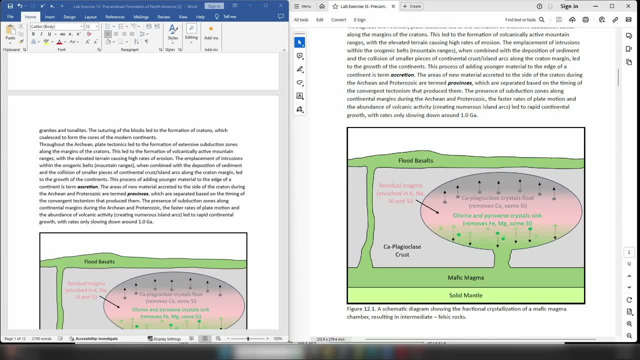 due to plate tectonics and as it's moving around the earth's surface due to plate tectonics, it is obviously going to collide with other younger rocks, so maybe younger island arcs, for instance. it's going to be moving around. it's going to come across an island arc. the two of them are going to. 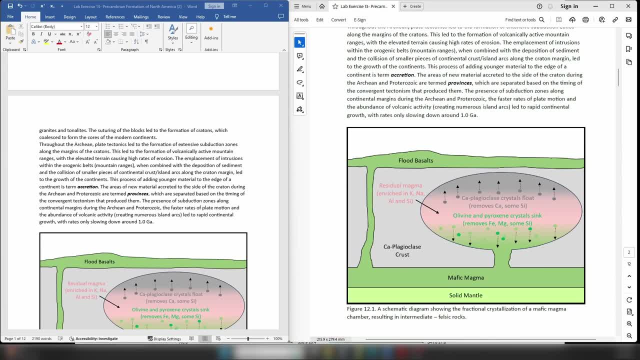 collide and the island arc is going to then stick, suture itself onto the sides of the craton and so, over time, what you're going to end up doing is you're going to end up adding more and more younger material along the edges of your craton. now, this is extremely efficient during. 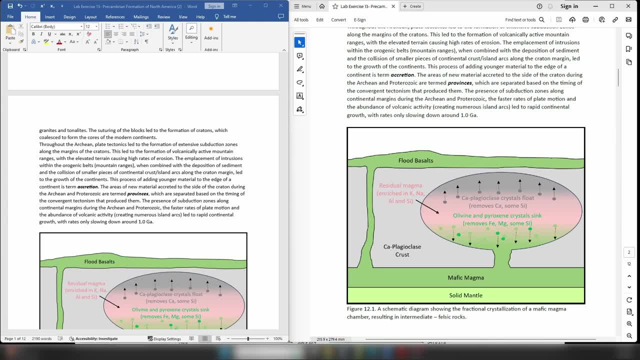 the archaean, because during the archaean it would seem that the margins of these content, these continental masses, were all active, and so this would mean that along the margins or all around the margins of these continental masses, you had a subduction zone, and so the fact you have this subduction zone is obviously going to mean that pieces of 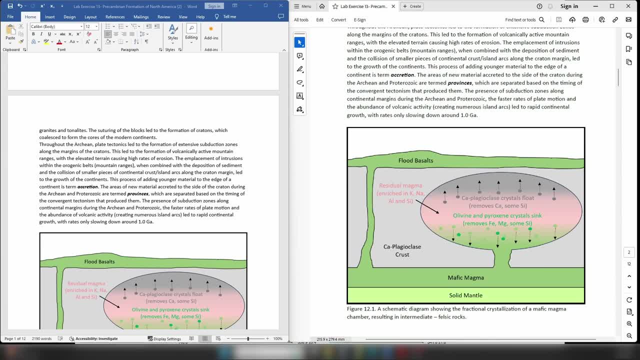 newer crust are going to be moving towards you and obviously that's going to result in the collision between these cratons and these- maybe island arcs, for instance, and other, maybe smaller, micro continents. it's also going to result in extensive mountain ranges and extensive volcanism, and this 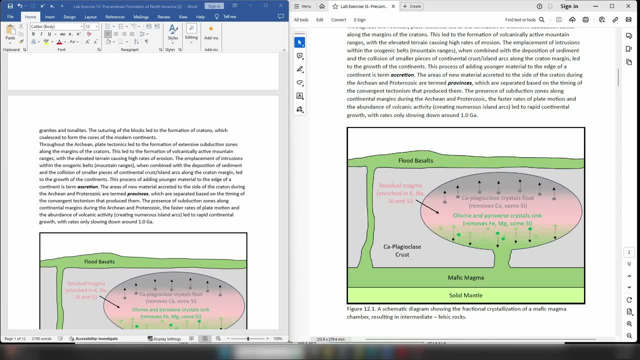 is important as well, because when you start having mountain ranges, well obviously that's bringing magma to the surface, so you're going to have a subduction zone and so the fact you have this surface, it's being erupting- erupted as lava, and that's forming new rocks which are also being 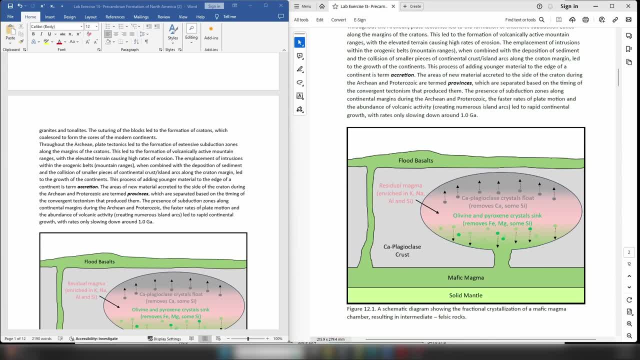 added, along the edges of our continental mass, we also have a situation where, because we are forming a mountain range due to these numerous collisions, we have topographically high land- and you probably remember that the highest rates of erosion are suffered by elevated terrain- so these mountain ranges will also begin to erupt, and so you're going to have a subduction zone, and so this is. 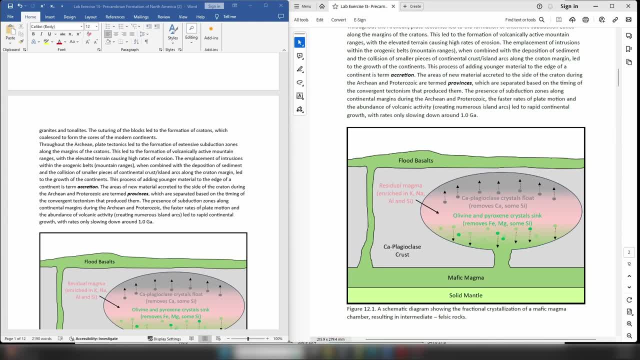 going to be eroded, producing quite large quantities of sediments, and this sediment will then be transported by rivers and it will be deposited along the coast of your continent. so you can begin to see how you will start to build up material along your continental margin. due to a 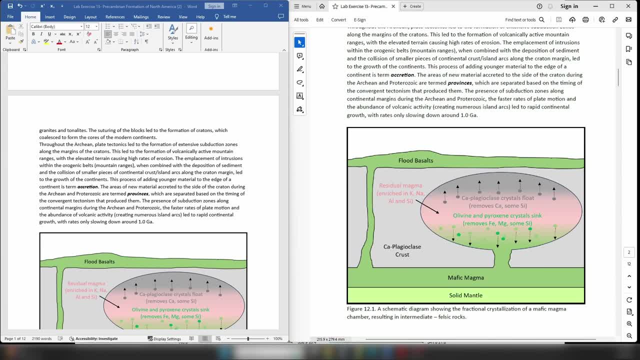 mixture of collisions, but also the as the result of volcanism and, most importantly, erosion of mountain ranges. so the areas where new material is being accreted or stuck to the sides of our craton during the archaean and protozoic are termed provinces, and a province is separated based on the timing of the. 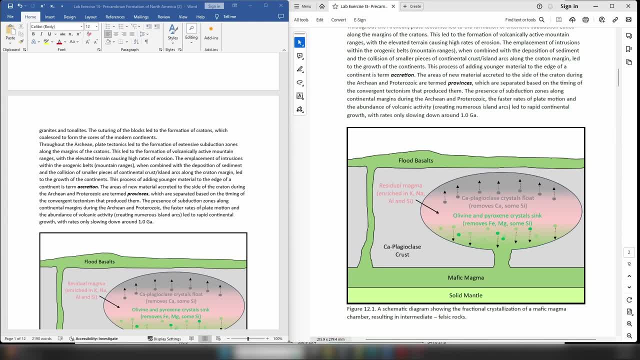 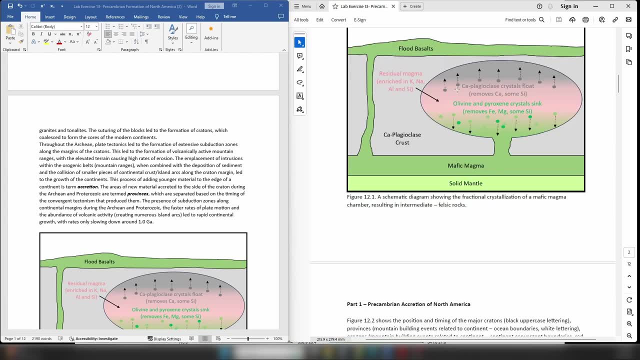 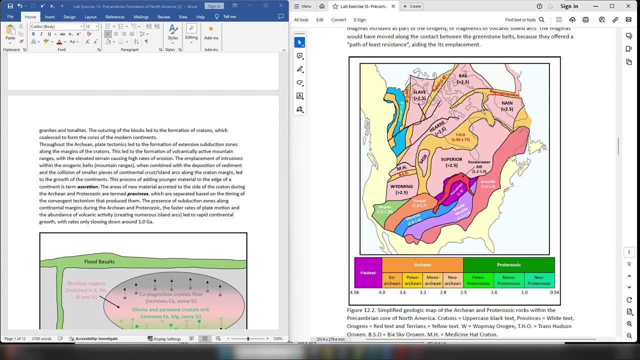 convergent tectonism that produced them. so the rocks that make up each province are the result of a particular tectonic event. so if we come down and we look at this diagram here, this diagram summarizes the main parts, the main cratons that make up the core of North America. so 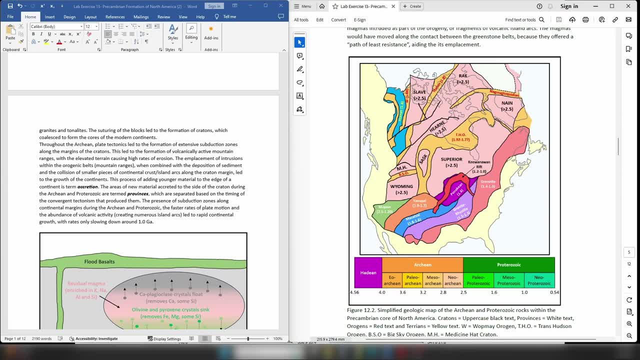 we have the superior province, we have the Hearn, we have the slave- uh, slave craton, we have Ray, we have the Sask, we have the Wyoming, we have the medicine hat. there's a lot of separate pieces of continental crust that have all come together to form the core of North America, and you can see in the case of 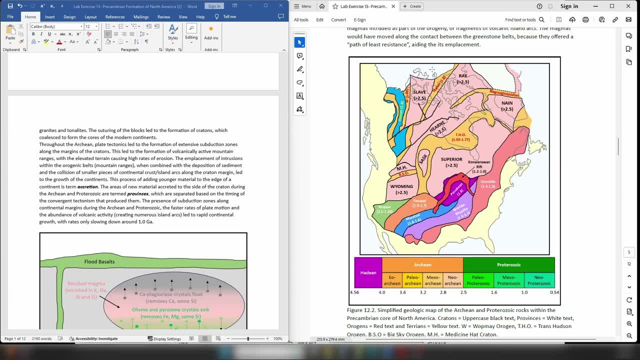 these two large chunks up here, so this chunk in the West and Northwest and this chunk which is situated in the South and East. they've both been stuck together by this large orogenic event here which is referred to as the trans Hudson orogeny, and so this is a very large mountain range that went and formed due to the 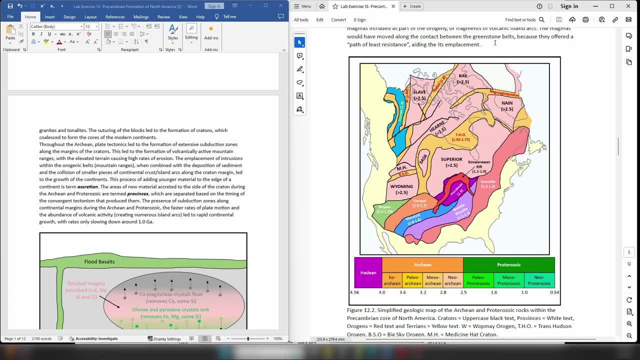 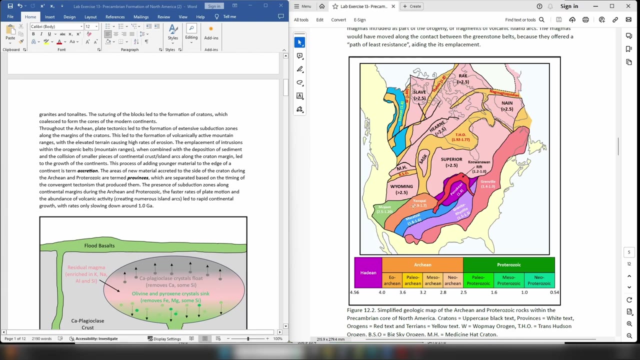 collision of these pieces of continental crust here and these pieces of continental crust here. so, once again, that would have produced a topographic high producing lots of sediment, and that sediment would have been eroded, transported by Rivers and then deposited along the margin of your rattle. so, um, you will notice that down here we also have a number of 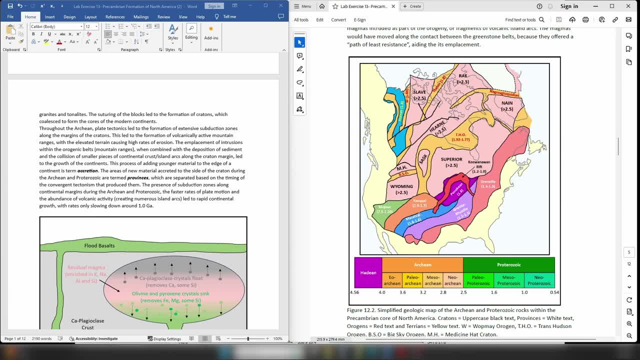 provinces. okay, so each of these regions down here represent different provinces produced by different tectonic events, so they will be a mixture of collisional events, so things will be on the side of our continent, but they will also be the result of tectonism, resulting in the formation. 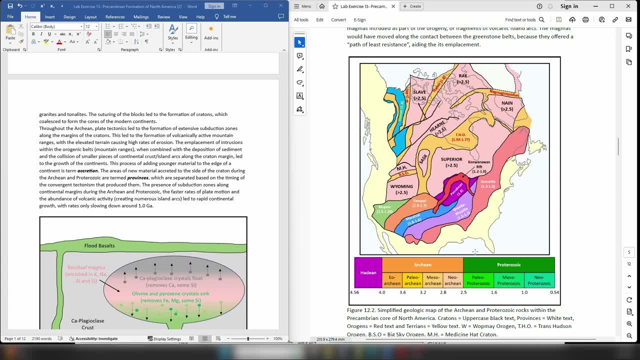 of new basins off the coast of our continental crust, our craton, and so if you imagine a situation, think of somewhere a little bit like Japan. so Japan is an active Island Arc which is produced due to a subduction Zone. now, behind Japan, you have a back Arc. 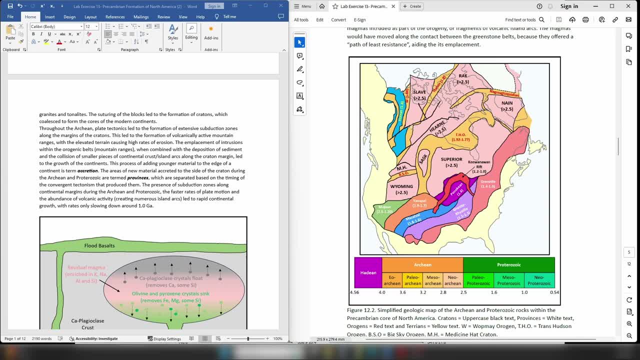 basin, which is a region of oceanic crust which separates the Island Ark from the mainland continent, in this case Asia, and so exactly the same thing will have been happening: you will have been having subduction along the edge of your continent, and this will have led to the formation 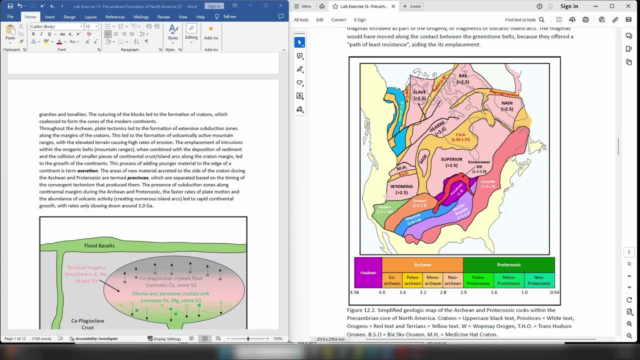 of island arcs which sit off the coast and behind these Island arcs, you would have had these Marine basins, these back Arc basins, and they will have filled with sediment from the erosion of the high up, the, you know, the parts of the craton itself. so the sediment which is produced by this erosion, 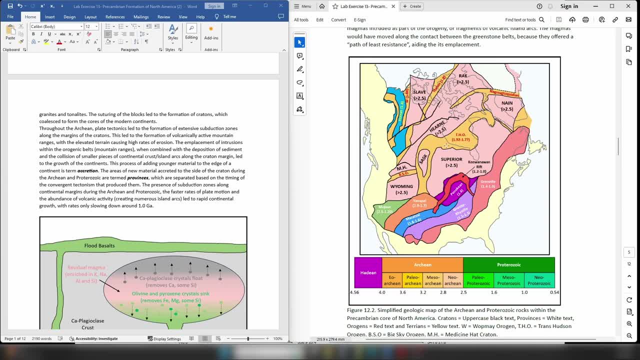 will be transported by rivers and it will be deposited into these back arc basins. now, eventually, plate tectonics says that a collision is going to occur and when that collision does occur, it's going to take that island, dark, and the back up basin and it's going to squish it between. 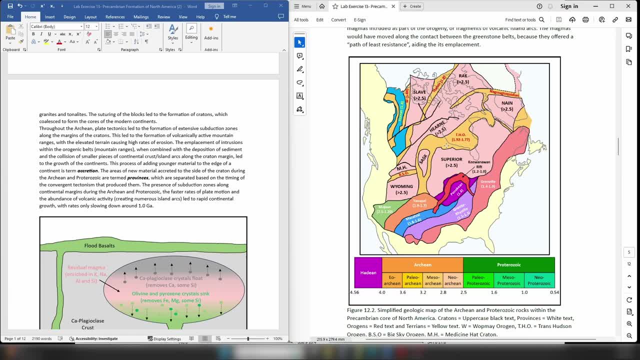 whatever. two pieces of continental crust are smashing into each other, and so this is going to result in the formation of these provinces. these provinces are a mixture of volcanic rocks. you're going to have intrusive and volcanic rocks associated with the island arc. you're also going to have a whole range of sedimentary rocks associated with the backyard basins. you're 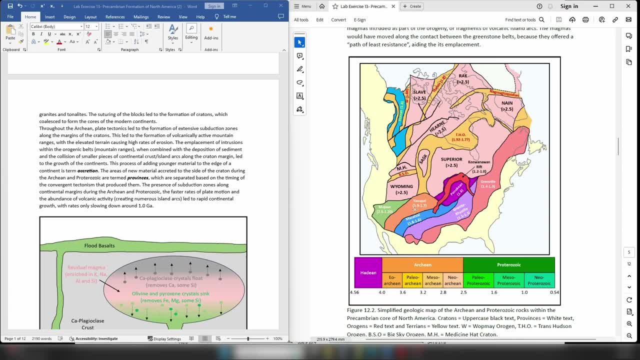 going to have lots of mud, stones, sandstones and maybe even some carbonates, and all of that is then going to be compressed and deformed by the collision itself. and because there's also a collision itself, the rocks are going to be crashed into each other, and they're going to be Ahora, and 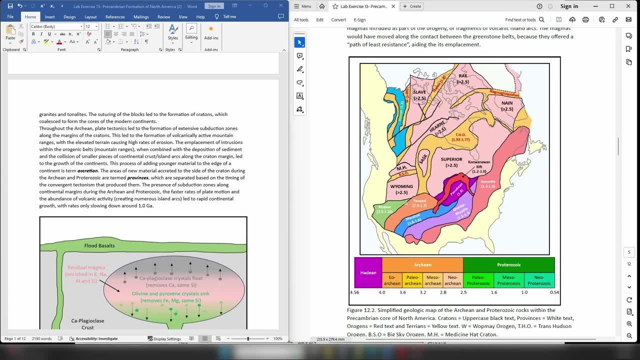 occurring. we are going to have an orogenic event which is going to result in further volcanism and also even more intrusions, and so each of these provinces down here, marked out by the white text, is going to be the result of the formation of these island arcs sitting off the coast and the 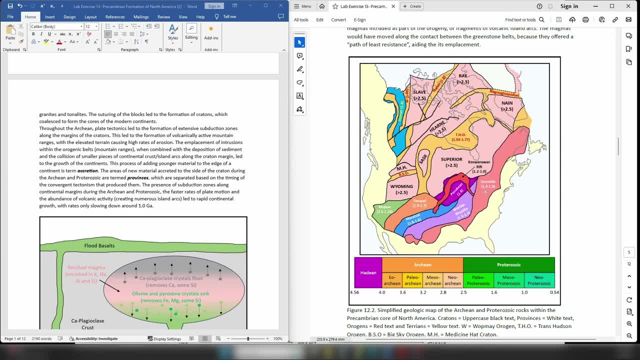 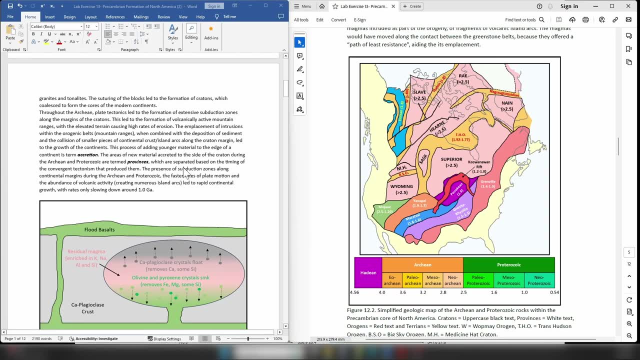 back arc basins and then the eventual closure and collision between the continent and the back arc basin and the island arc. Okay, so in terms of how often these collisions were occurring, we're not totally sure because it's pretty difficult to interpret, you know, the geologic evidence, because 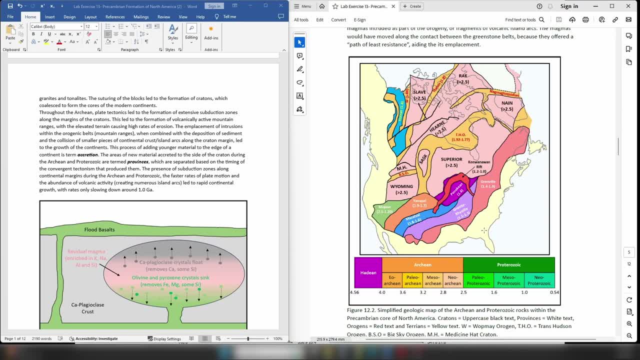 a lot of these rocks have been metamorphosed, sometimes to very high levels, so original textures and original features have been lost. We do, however, know that, due to the faster rates of plate motion in the Archean and in the early prognostications, 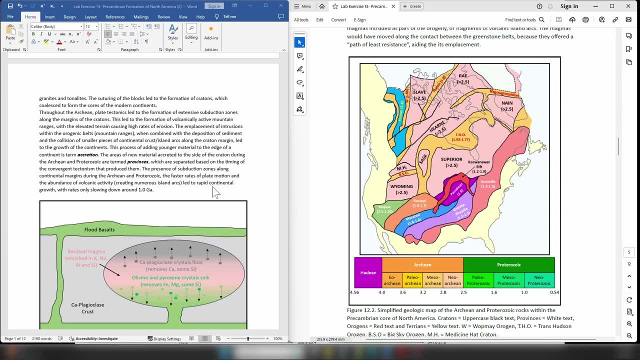 we know that these collisions will have been happening regularly, you know, quite frequently. and we also know that the rate of these collisions began slowing down after about 1 billion years ago, and that seems to be when things are starting to slow down, become, you know, plate tectonics is becoming more controlled, more like the plate tectonics we know. 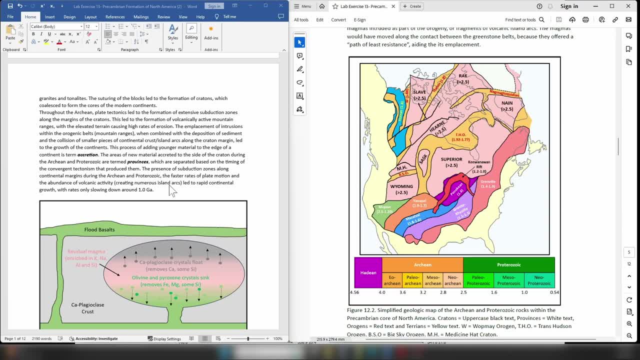 now. So this is a good place to stop. so please get up, have a walk around, go and get yourself a glass of water and return for part two.